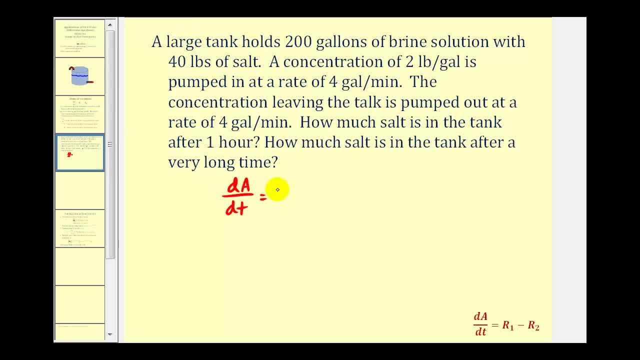 So, using our differential equation, dA, dt equals R sub one minus R sub two. So we want to start this by finding R sub one, the rate at which A of T is entering the tank, and R sub two, the rate at which A of T. 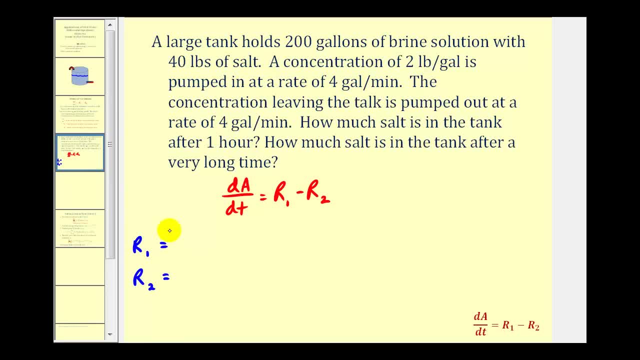 is leaving the tank. To find these we'll have to multiply the concentration times, the rate. So for R sub one, notice how there are two pounds per gallon. that's being pumped in at four gallons per minute. So we need to find this product. 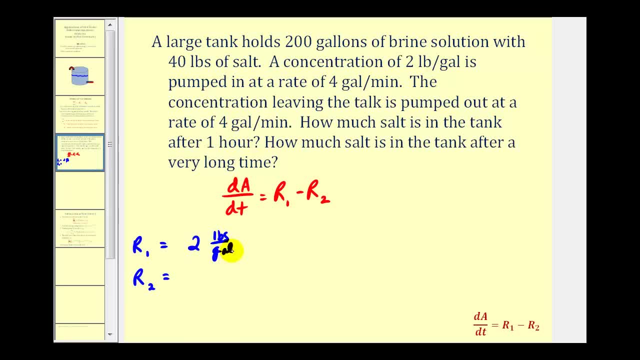 So we have two pounds per gallon times four gallons per minute. Now, the reason I'm writing this in fraction form is so that we can easily see that the units of gallons simplifies out. therefore, R sub one is going to be eight pounds per minute. 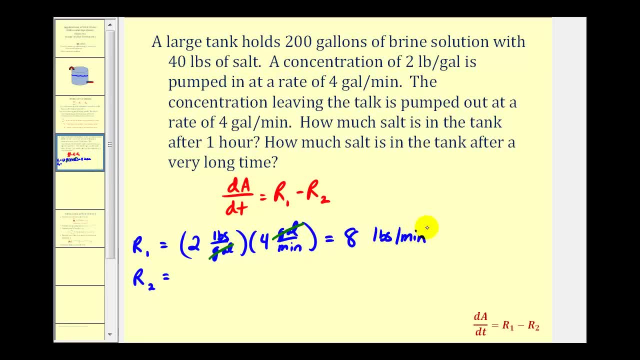 Now R sub two is going to be a little bit trickier. We're going to have to write an expression for the concentration because it's changing as the mixing occurs. Notice how we start off with 40 pounds of salt per 200 gallons, but the 40 is changing. 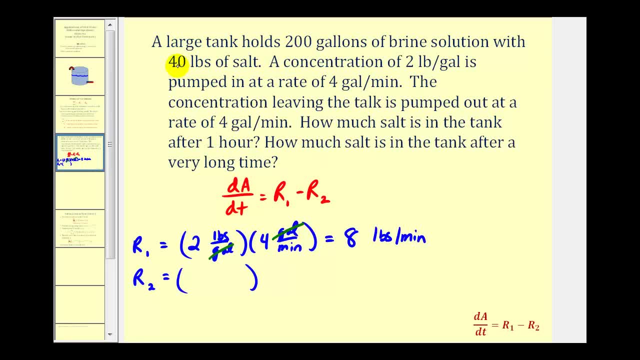 so we can't use that for our concentration. We have to use an expression, so we'll use A, where A is the unknown divided by 200, and that's two, and this would be pounds per gallon, And then the rate is the same as four gallons per minute. 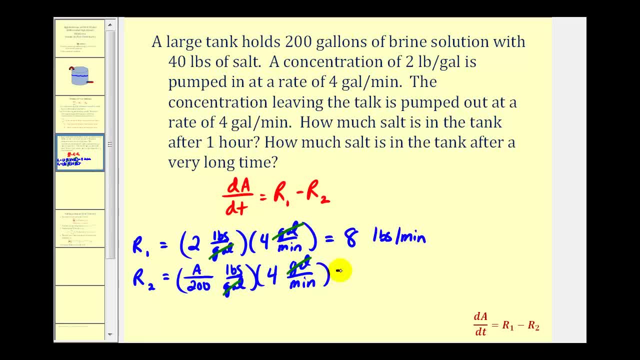 You can notice how gallons simplifies out. so we're going to have this would be 4a over 200, and this would be pounds per minute. But this does simplify: 4 over 200 is 1- 50th. 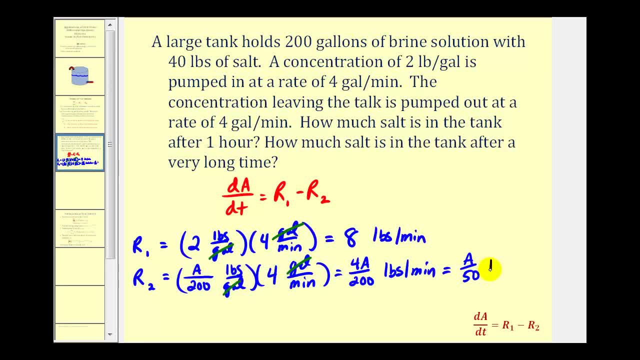 so we have a divided by 50 pounds per minute. So our differential equation would be: dA. dT equals eight minus a divided by 50. Well, this is actually a linear first order differential equation which we can solve by using an integrating factor. 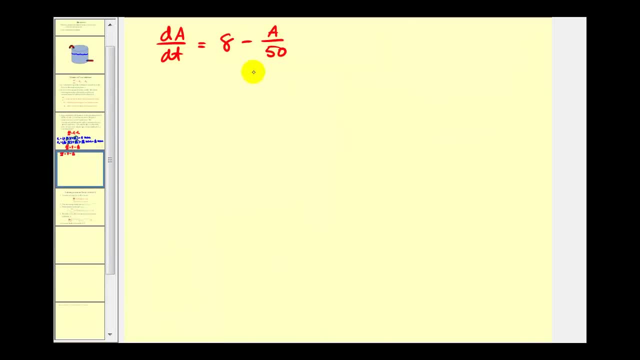 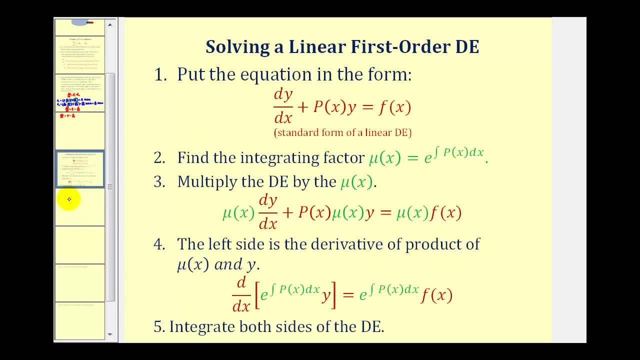 Let's go ahead and set this up on the next slide. So just to review: if we have a linear first order differential equation, then we're going to write the differential equation in standard form or this form here and then we're going to multiply everything. 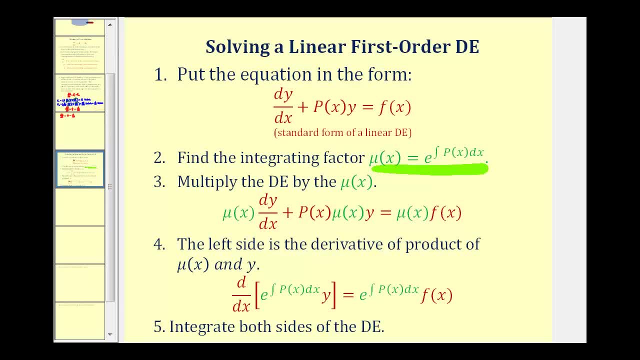 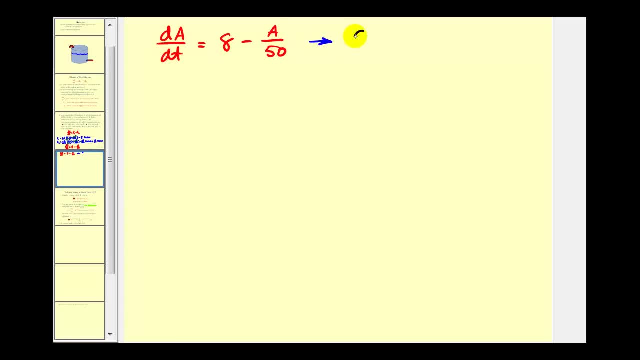 by our integrating factor, which is given here. So you may want to pause the video here if you need this review. So I'm going to go ahead and rewrite this in standard form. so we'd have dA dT plus 1 50th a equals eight. 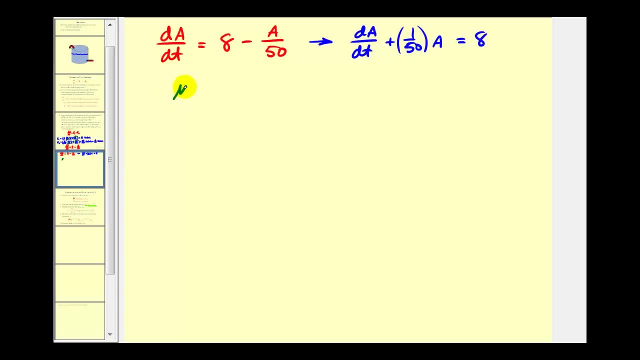 So in this form we should recognize that the integrating factor mu of T is going to be equal to e raised to the power of the integral of 1, 50th dT. So this is just going to be e to the T divided by 50th power. 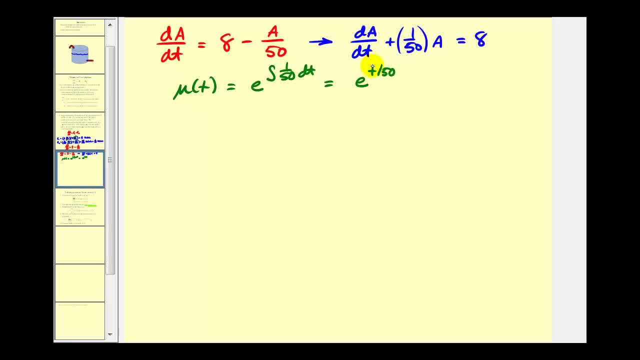 Now we're going to multiply everything in this differential equation here by this integrating factor. So we're going to have e to the T divided by 50, dA, dT plus 1 50th e to the T divided by 50 times a. 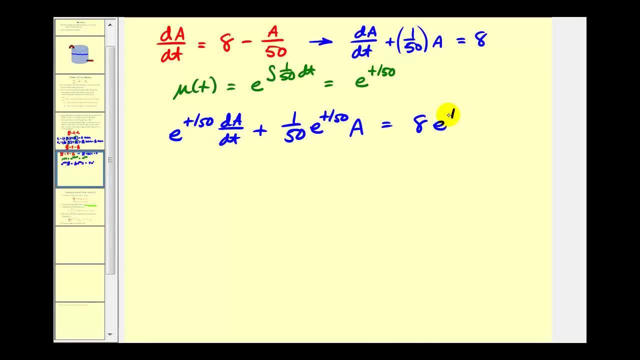 equals eight times e to the T divided by 50th power. Now, once we multiply everything by the integrating factor- remember, the left side of this equation, or this side here, is equal to the derivative of the product of the integrating factor and our function, a. 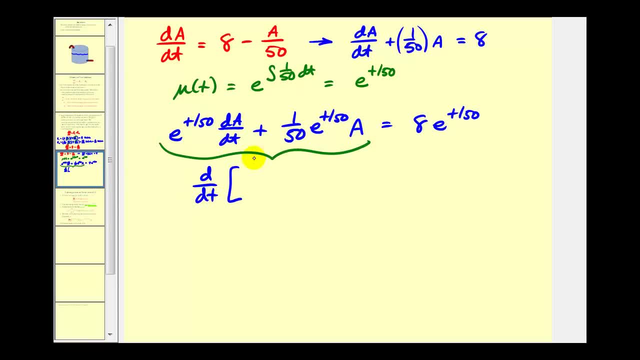 So the derivative with respects to T, with the integrating factor which is e to the T divided by 50 times our function, a. So if the left side is equal to the derivative, then it must also equal the right side. So we'll set this equal to 8e to the t divided by 50th power. 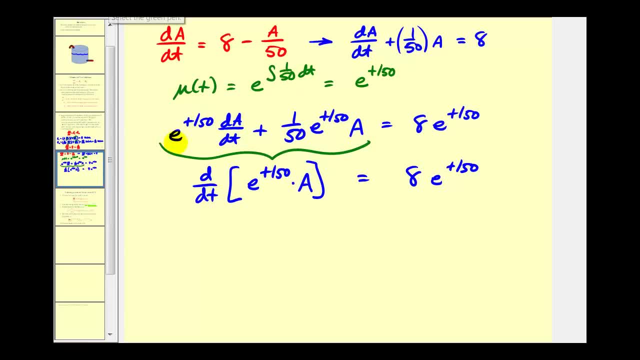 And now we'll integrate both sides of the equation with respects to t. On the left side, the derivative and integral undo each other, So we're left with the exponential times a must equal. Over here we have to integrate using u substitution. 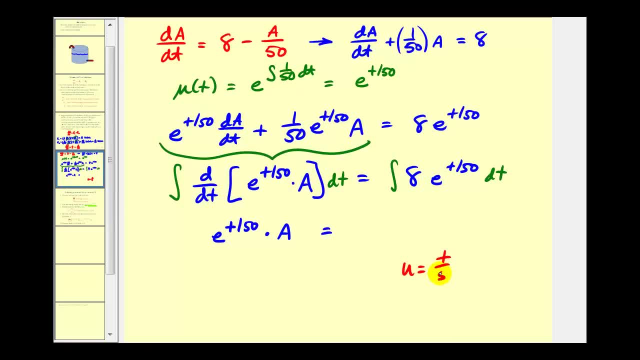 So notice here: if we let u equal t divided by 50, then du is equal to 1 50th dt. So that means 50 du is equal to dt. So when performing the substitution we're going to have an extra factor of 50. 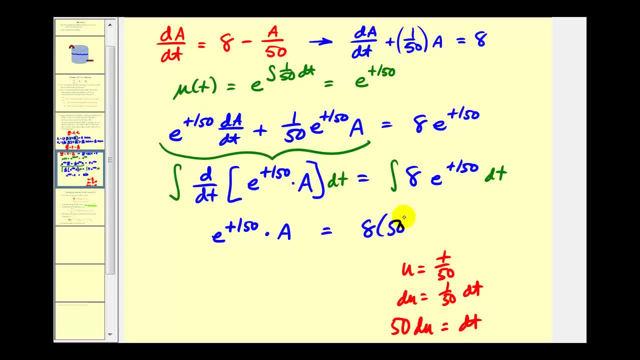 So the anti-derivative will be 8 times 50 times e to the u or e to the t divided by 50.. And then, of course, plus our constant of integration. Okay, now, our goal here is. okay, now our goal is to solve this for a or a of t. 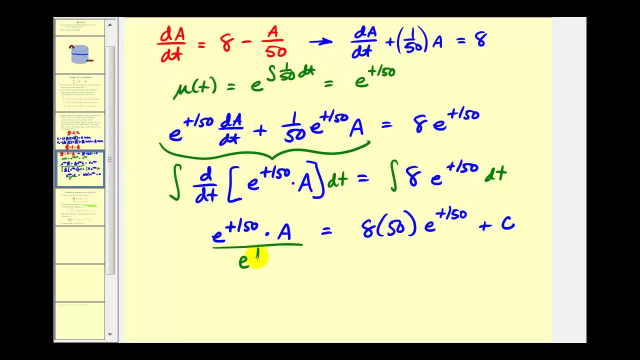 So now we'll divide both sides by our exponential. So on the left side, simplify this to a or a of t. On the right side, these exponentials simplify to 1. So we have 400.. And here we can just write this as plus c. 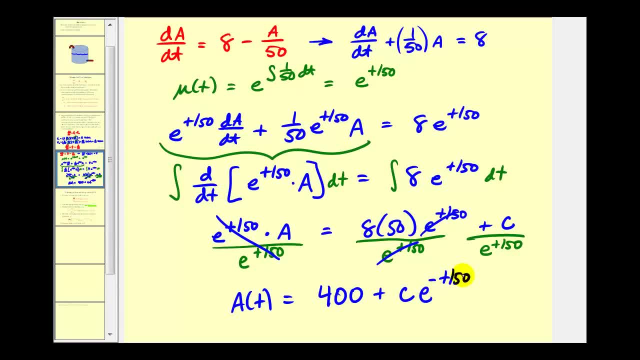 Times e to the negative t divided by 50th power. Now that we have the general solution, we can find the particular solution using the initial condition that a of 0 is equal to 40, because there's 40 pounds of salt to begin with in the 200 gallons. 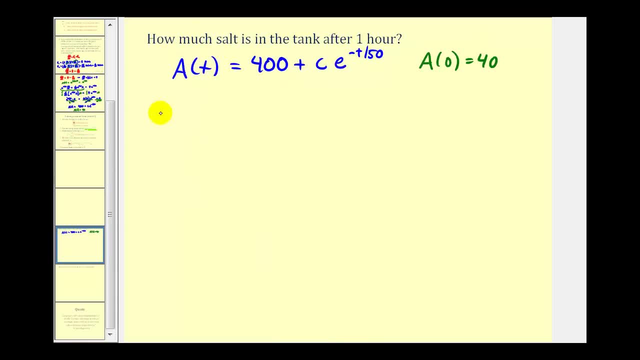 Let's go ahead and do this on the next slide. Okay, so if a of 0 equals 40, we'll replace t with 0. We would have 400 plus c, times e to the negative t, Times e to the 0,, which is equal to 1.. 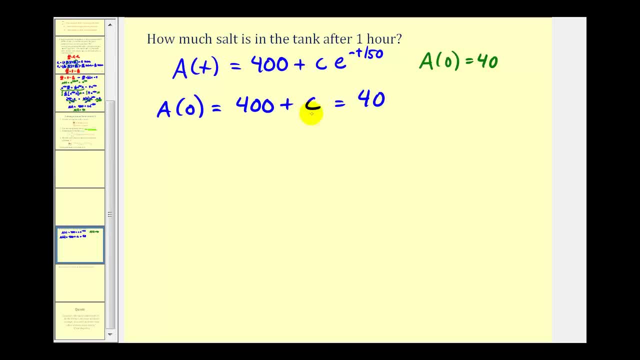 So this is just c. This must equal 40.. So we'll subtract 400 on both sides, So c must equal this would be negative 360.. Therefore the function that models the mixing solution is: a of t equals 400 minus 360 times e. 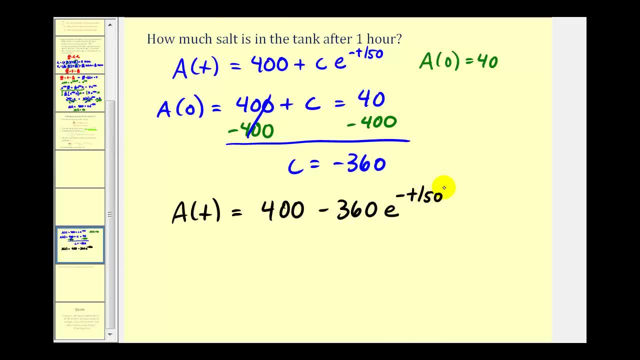 to the power of negative t divided by 50. And now we're going to do this, And now we can determine how much salt is in the tank after 1 hour. but we need to be careful here, because t is time in minutes. 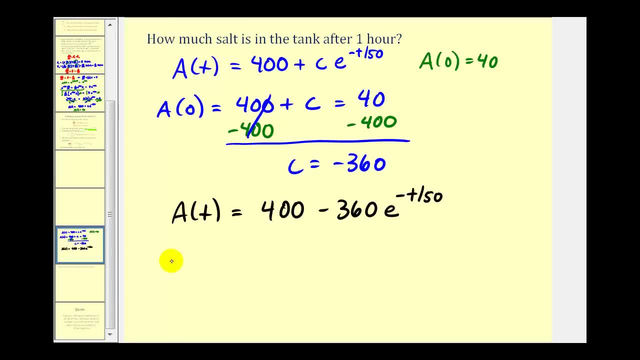 Therefore, for 1 hour we have to find a of 60, not a of 1.. And we know this because the initial flow rates were given in gallons per minute. So our exponent here would be negative 60 divided by 50.. 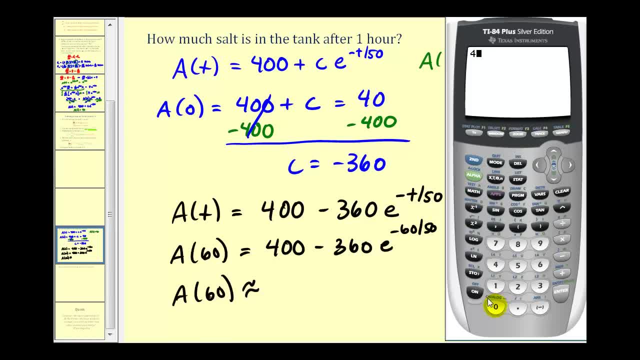 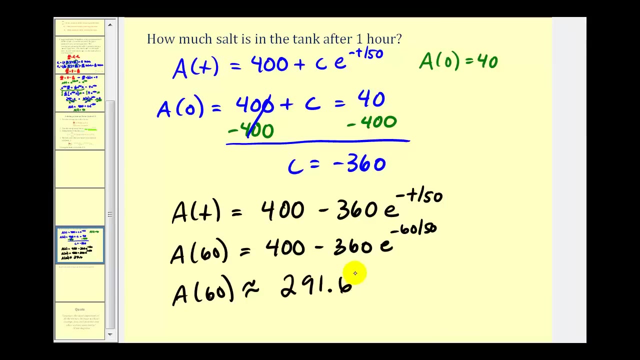 And now we'll go to the calculator. So there's approximately 291.6 pounds of salt in the tank after 1 hour. And now for the last question: how much salt is in the tank? after a very long time we can answer this.